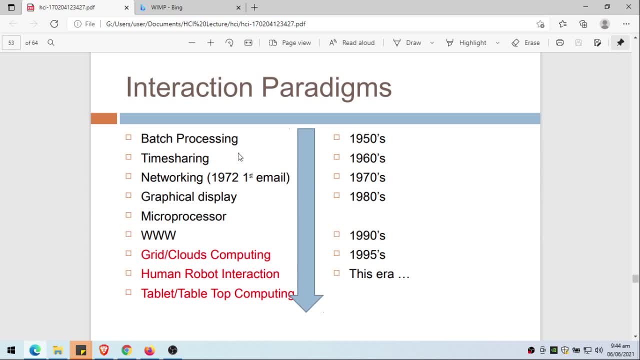 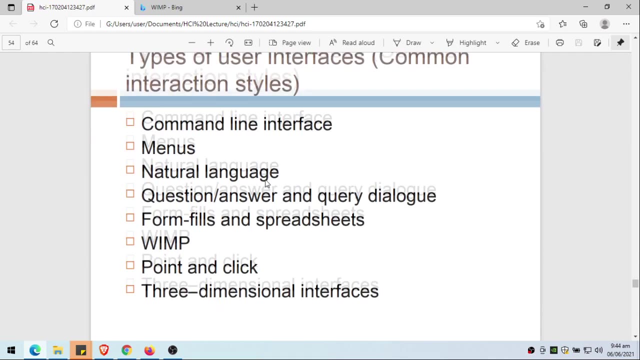 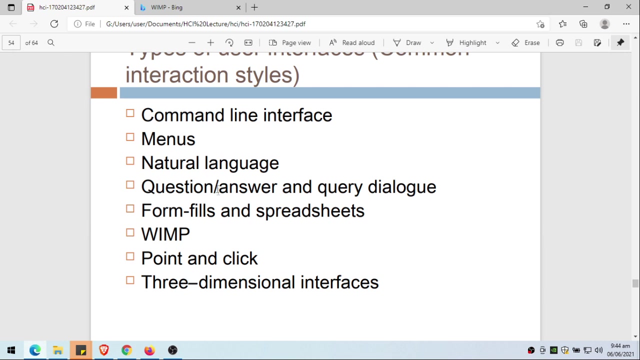 And so, as we notice that as technology progress, the interaction between human and computer is actually changing, So here are some types of user interfaces and these are the common interaction styles. So we have the command line interface, Menus, Natural language, Question answer or query dialogue. 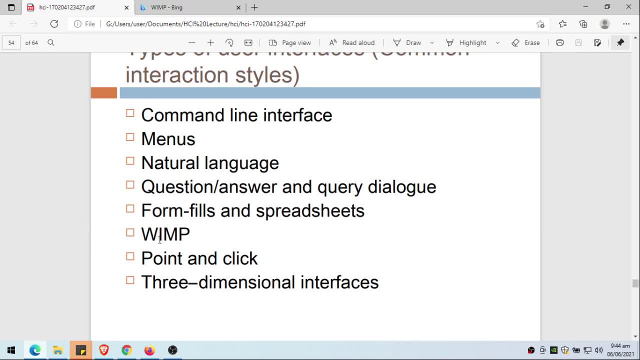 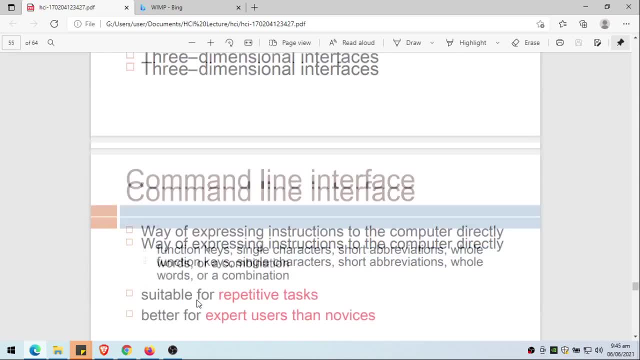 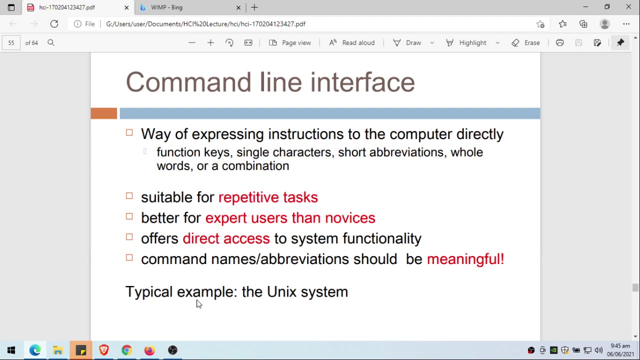 Form fields and spreadsheets. We have the WIMP Or W-I-M-P, Point and click, And we also have three-dimensional interfaces. Let's take a look at the command line interface, So way of expressing instructions to the computer directly. 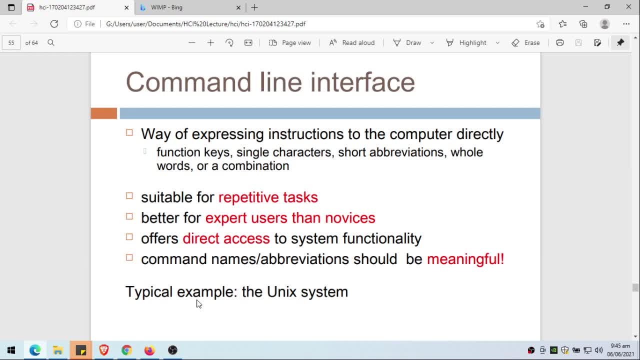 So function keys, single characters, short abbreviations, whole word or a combination. So it is where we actually type the command itself. So these are suitable for repetitive tasks and it is better for expert users than novices, Because of course you have to more or less be familiar with all the commands and you should have memorized the commands that you'll be using. 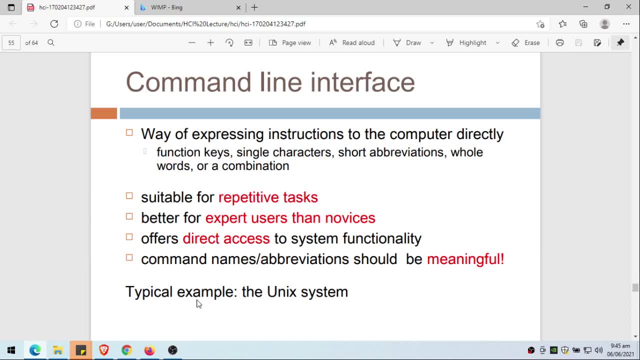 And it offers direct access to system functionality. Then command names, Then command names- abbreviation should be meaningful. So if you have used, for example, the old PC DOS or Microsoft DOS, MS DOS, Then that is an example of a command line interface. 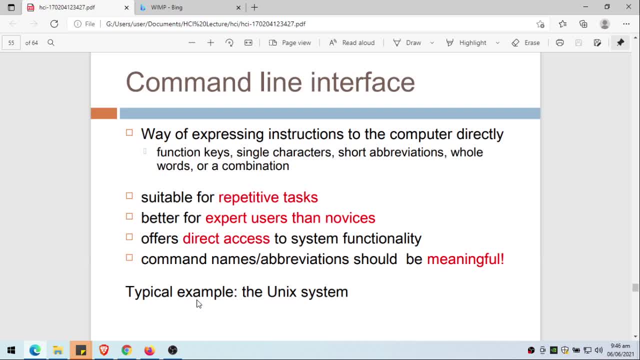 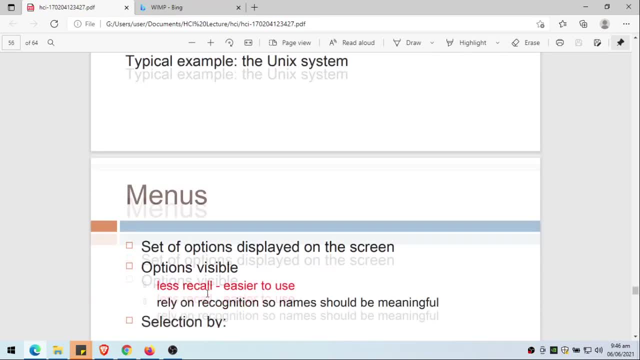 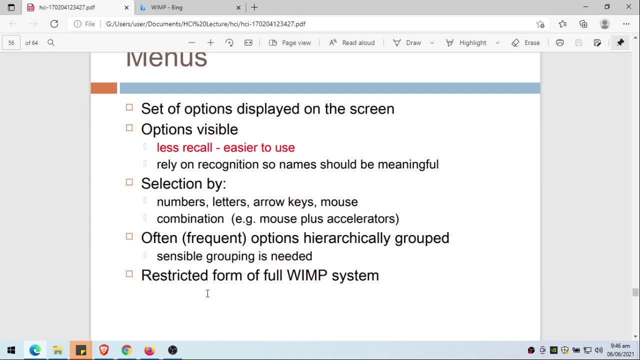 Also. the typical example is the UNIX system. So the UNIX system is making use of command line interface. Then we have menus. So a menu is a set of options Display Played on the screen. So options are always visible or visible. So less recall is easier to use because you can view the options, especially as compared with a command line interface. 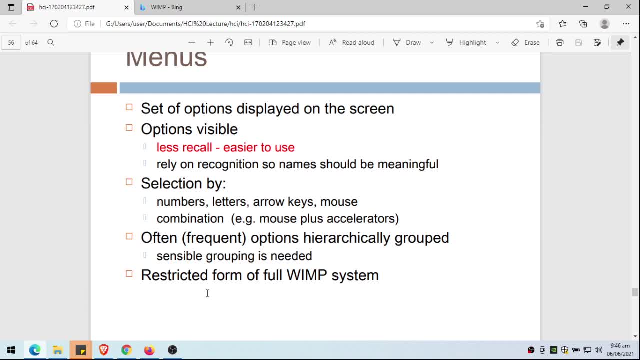 So rely on recognition. So names should be meaningful. So that means if you, if you can see the option, then you should be able to recall or know the use of the particular option. So the selection: We can use numbers in selecting letters, arrow keys or mouse, or maybe even combinations of this. 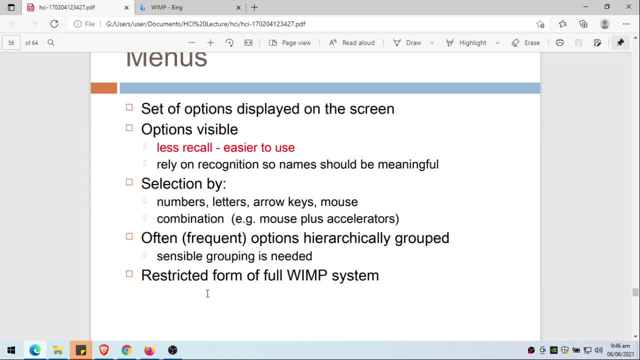 So often or frequent, options are hierarchically grouped, so sensible grouping is needed. So you have to group the options, especially if you have a long menu. because if you don't group your options or maybe sensibly arrange your options, Then it would be hard for the user to select the option. menu option. 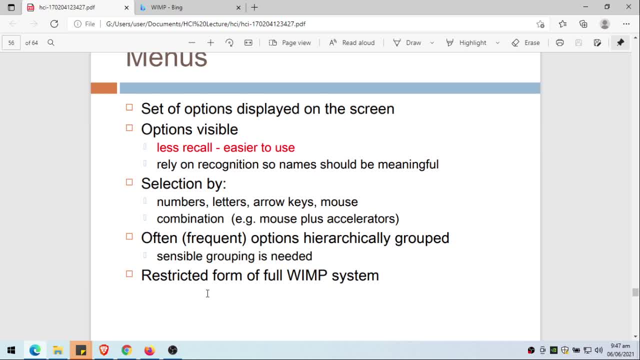 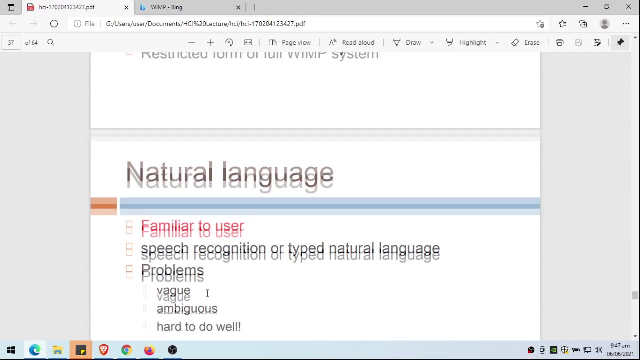 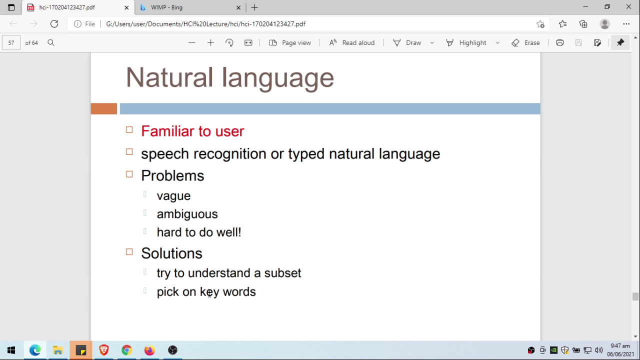 So restricted form of full WIMP system. So later on menus are also used in especially graphical user interface, But there are also menus for text interfaces. Then we also have the natural language. So the natural language seems familiar to the user because of course it is the natural language. 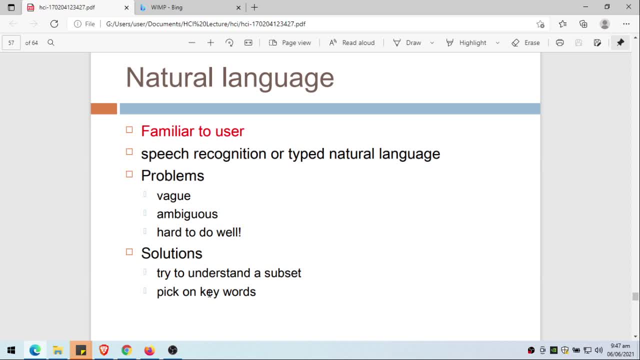 So I see if you're just talking naturally to the computer. So it's speech recognition or type natural language. So in most cases the natural language will use speech recognition or sometimes you can also type the natural language. So the problems: sometimes it can be vague or ambiguous. 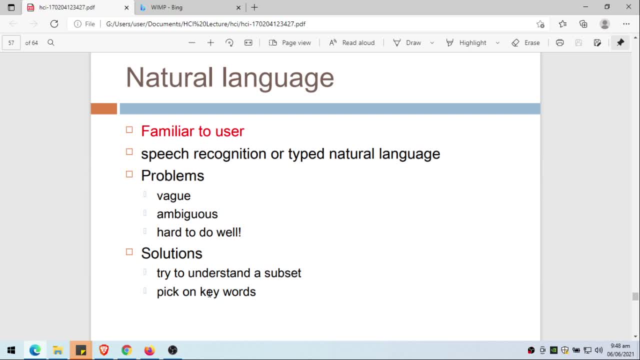 So let's say, for example, that Maybe there are words that can have dual meaning, So sometimes it can be hard to do well. So solutions: we try to understand a subset or pick on keywords. So that is how computers make natural language more effective. 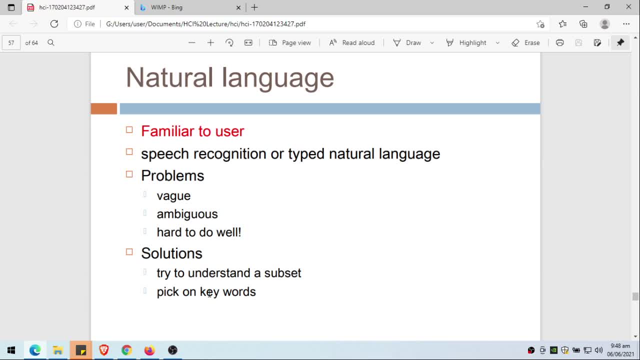 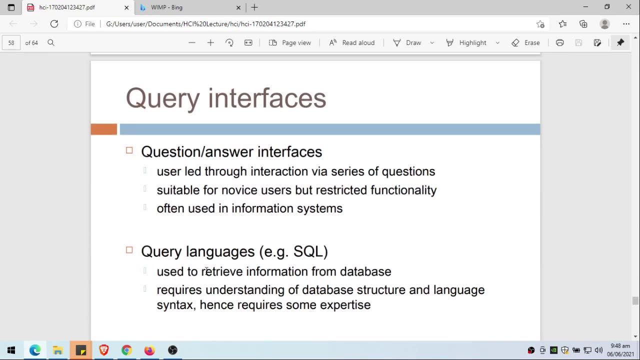 And, up to this point, although we already have natural language is gaining popularity. Of course it is natural, yet perfected. we also have what we call the query interfaces. so these are question and answer interfaces, so user led through interaction by a series of questions. so if you have, if you're familiar with installation wizards, these 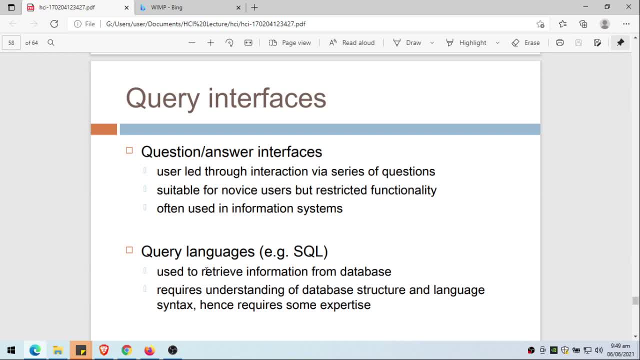 are examples, maybe, of question and answer interfaces: so suitable for novice users, but restricted functionality, so what? what the user can only do is what is placed in the screen and often used in information systems. we also have query languages like SQL or SQL. these are used to retrieve information from 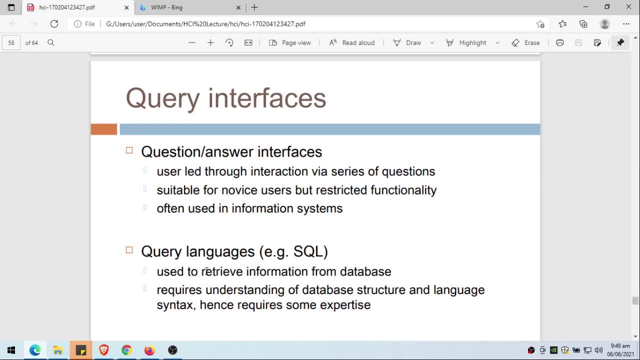 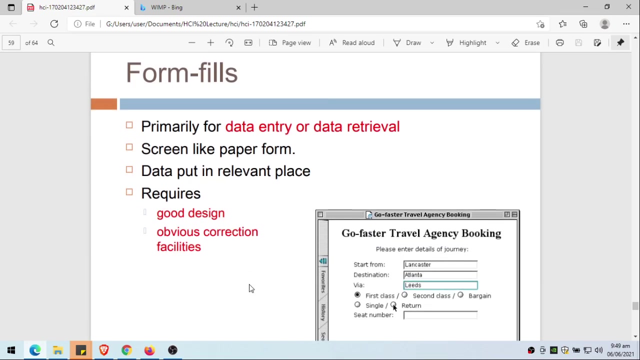 database requires understanding of database structure and language syntax. hence requires some expertise, especially if you're using the command line interface of SQL. but there are actually graphical, graphical applications where you can query a database, like QBE for example, that is used by Microsoft Access, then form fields, so primarily for data entry. 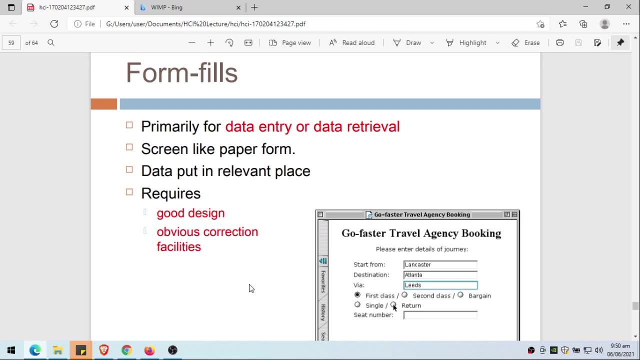 or data retrieval. so it is a screen like paper form. so, as you can see here on our screen, this is an example of form and we can type data. that's why it's called form field. so data put in relevant places and requires good design, because if the design is bad it can confuse the user, and obvious correction facility. so 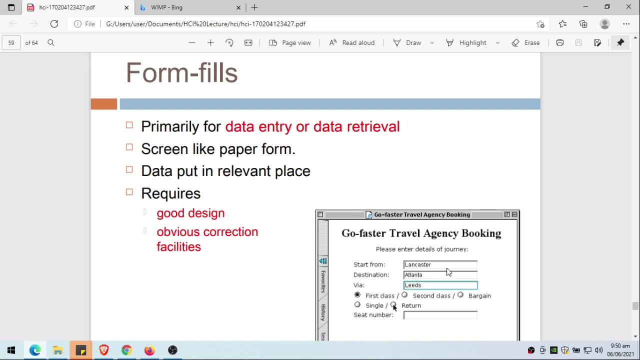 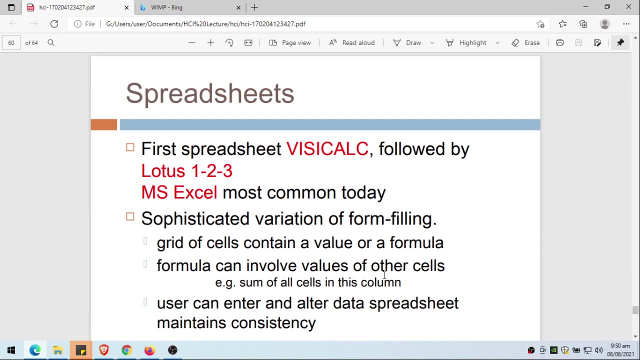 the user should be able to correct errors. and again, we'll be discussing more of these as we go on with our with this course. so thank you for watching and we will see you next time. the HCI course Spreadsheets. so first spreadsheet is the VisiCalc, then 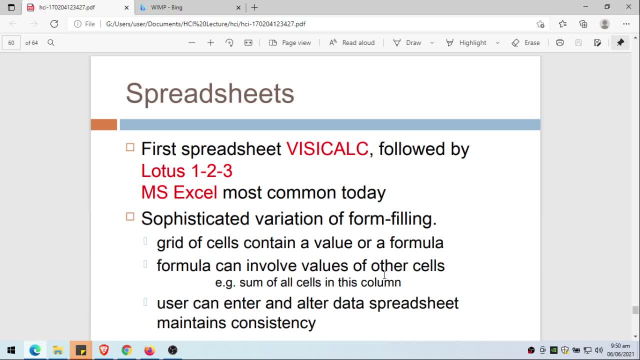 followed by Lotus 1-2-3, and Lotus 1-2-3 was actually very popular during the 80s and maybe up to the mid 90s, but now I think the most popular and the most common spreadsheet is the Microsoft Excel, so it's a sophisticated variation. 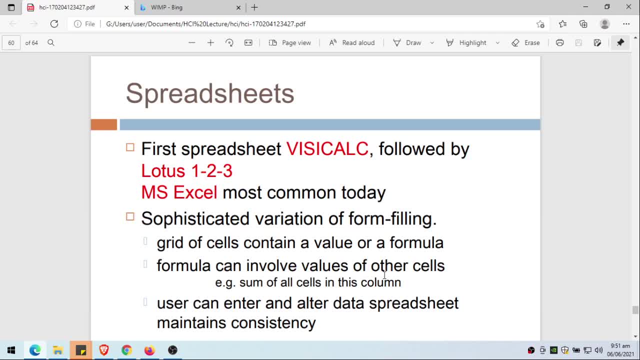 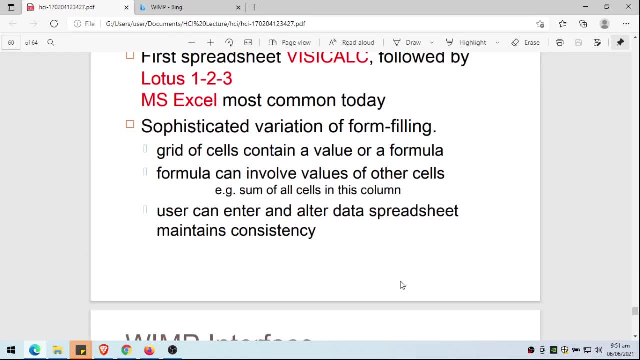 form filling, because we use grids, or grid of cells contains a value or a formula, and formula can involve values of other cells. so if you're familiar with Excel, you know how to do this. let's say, for example, if you want to get a sum of different cells, so in this, in a particular formula, you have to reference. 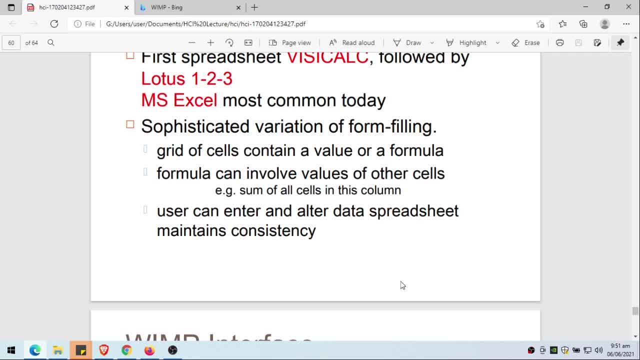 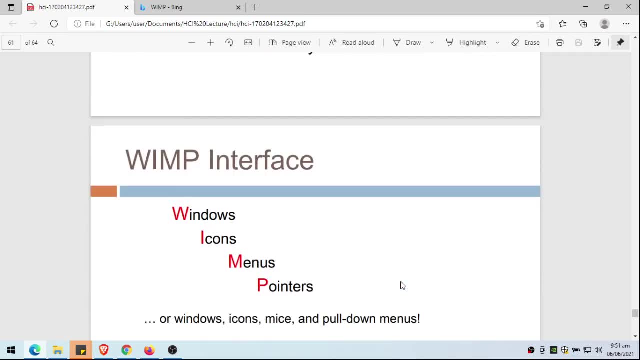 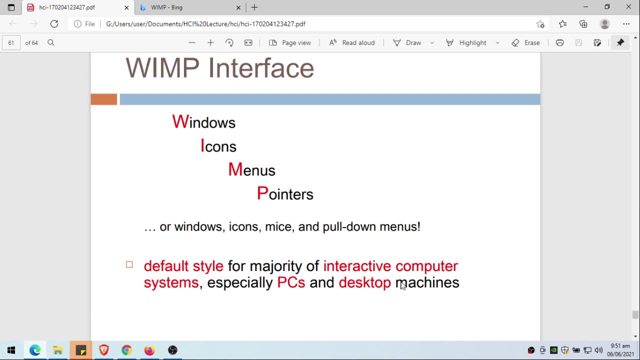 several cells so user can enter and alter data. spreadsheet, also mentioned, contains consistency. then we have the wimp interface or the windows icons, menus or pointers, or some we'll call it windows icons, mice and pull down menus. but basically this is a graphical user interface, so default style for majority of interactive computer systems especially. 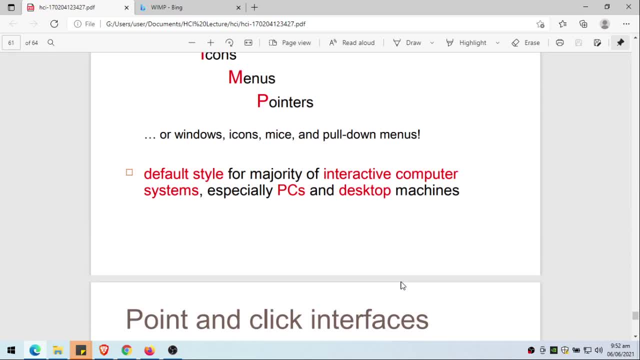 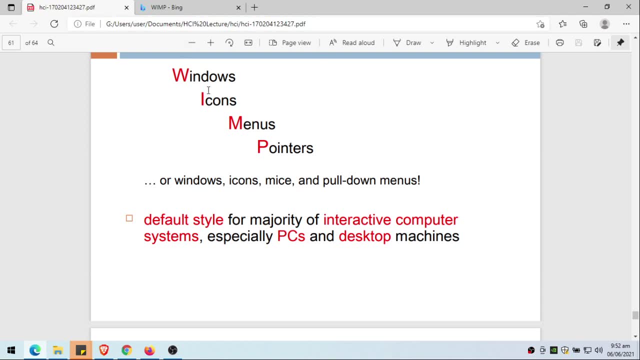 pc's and desktop machines. so the windows, your our operating system and, of course, what you're on my screen now is an example about windows icons, menus and pointers. as you can see, this is a. the browser is a window, so i have here several icons. you can see also my if i click on this. where 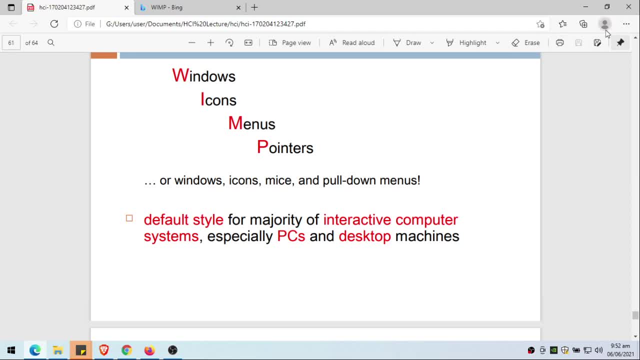 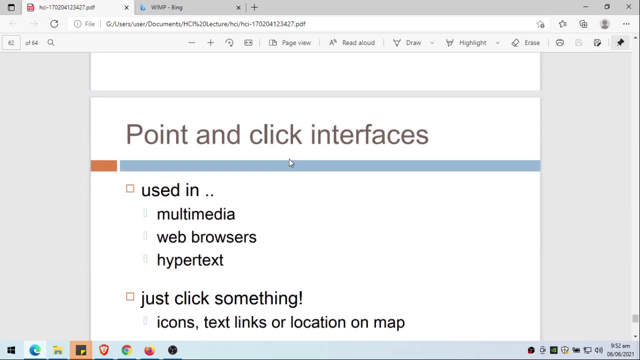 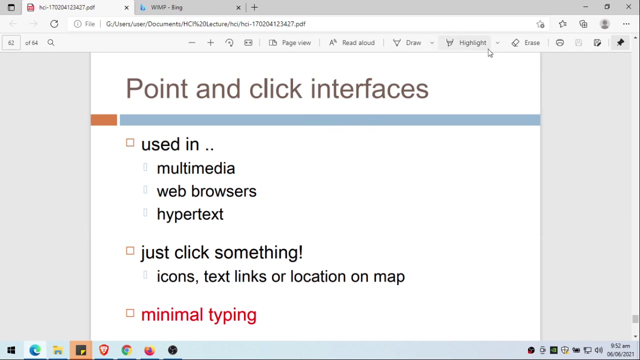 so, for example, this happen for this one. so that's an example of a menu and of course you can see my mouse pointer. so this is an example of wimp, or wimp. then we also have the point and click interfaces, so used in multimedia web browsers, hypertext. so we have pointer and we can click on anything here. so 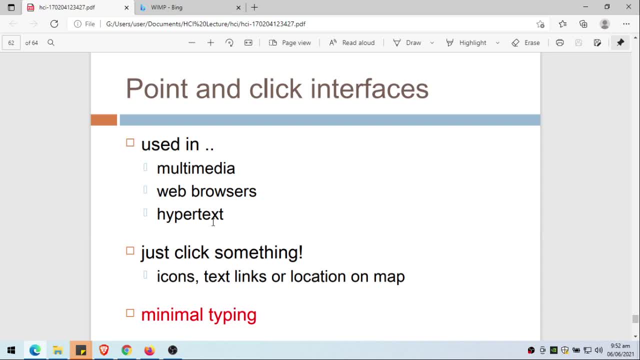 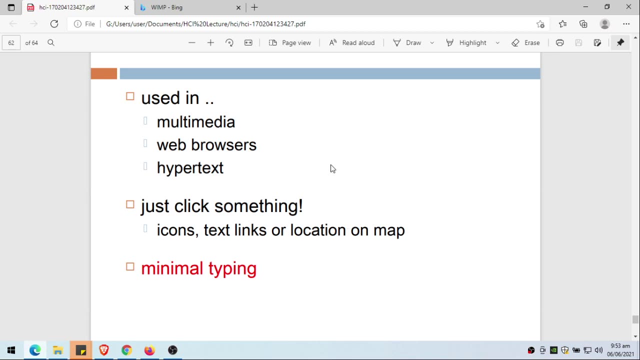 hypertext. i know you're familiar with hypertext, especially on web browsers. so just click something and icons, text, link or location and them up. so these are point and click, some minimal typing here. um, we almost make use of the pointer or point and click all the time. then we also have the 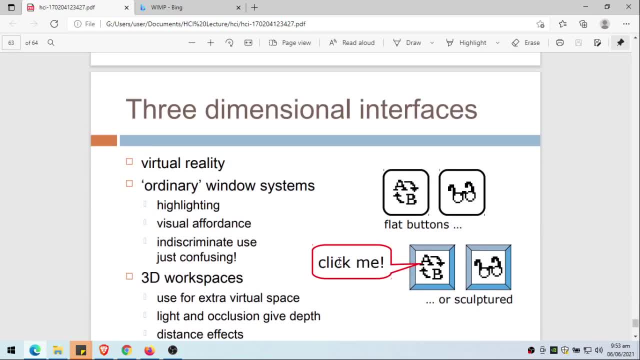 three-dimensional interfaces, and one example of this is, of course, virtual reality, wherein you can see a 3d representation of the reality or the real world, and also ordinary windows system can use highlighting visual affordance, discriminate use, just uh, we can have, for example, some sort of 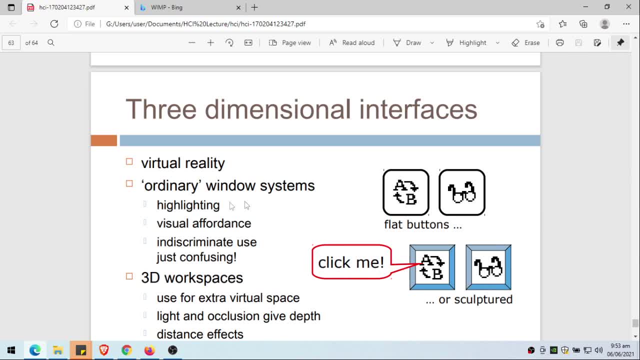 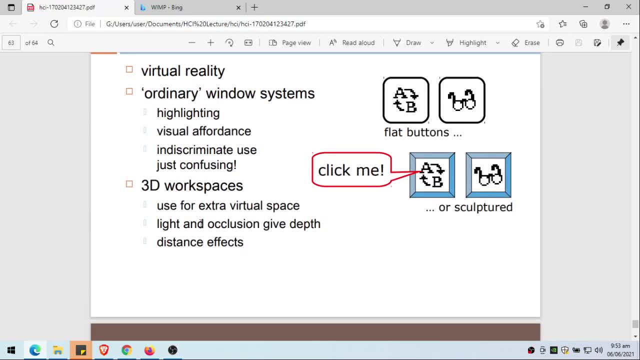 this sculptured, so it's an example of a 3d ordinary window system, but if it is used indiscriminately it can be confusing. then we also have 3d workspaces used for extra virtual space. light and occlusion give depth and distance effects. so again, i think this is similar to virtual reality. 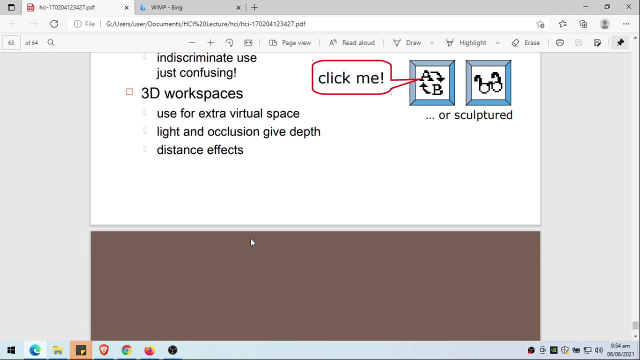 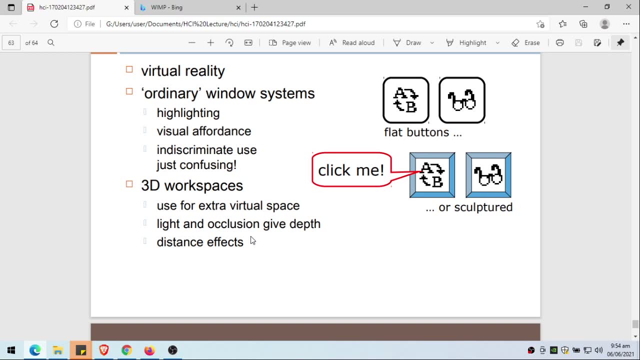 and actually we may have more of this interaction, but for now these are, as i've said, just a tip of the iceberg when it comes to computer interaction. so for now, i will end my lecture and, uh, i will be discussing more. we'll be discussing more of these in a while. over next lectures. so thank you very much.